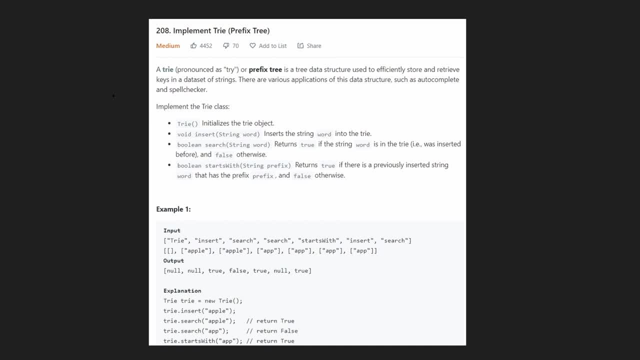 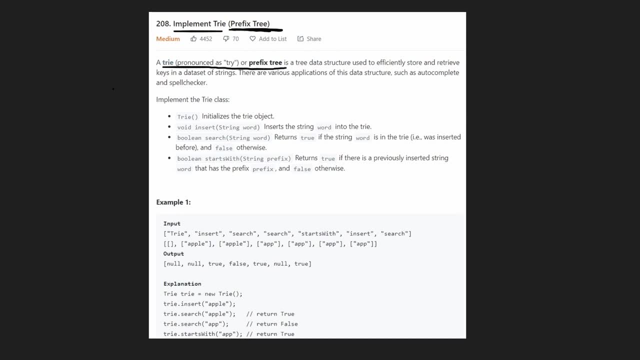 Hey everyone, welcome back and let's write some more neat code today. So today let's solve, implement try, aka a prefix tree. So a try or a prefix tree is a special type of tree and it's used to efficiently store strings, and the applications are some stuff like autocomplete. 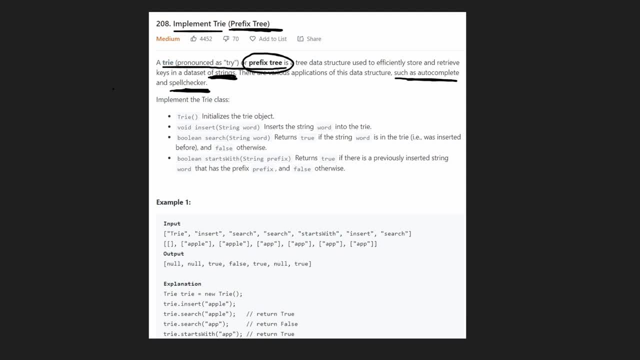 and spell checker. The reason is because the prefix tree allows you to efficiently filter and search based on prefixes. So let's look at the actual implementation of it. So we're going to have a object- That's what we're going to be doing this time- a try object, And our job is to 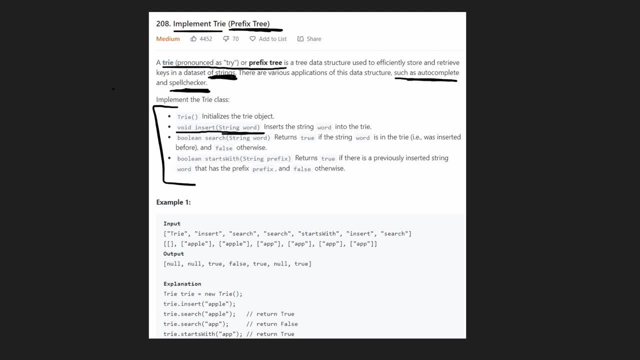 fill in three functions. The first function is going to be inserting a word into the try. The second function is going to be searching for a word in the try to see if the word exists. And the third function is going to be to check if there is a word that starts with a given. 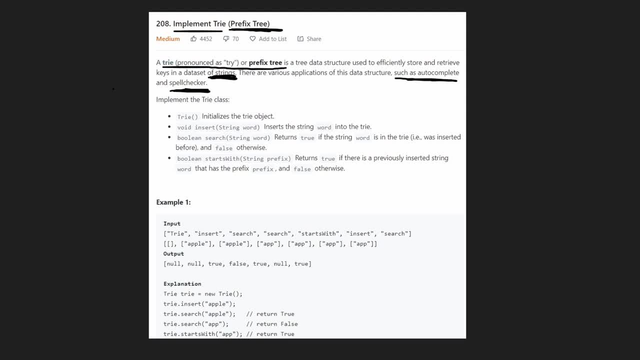 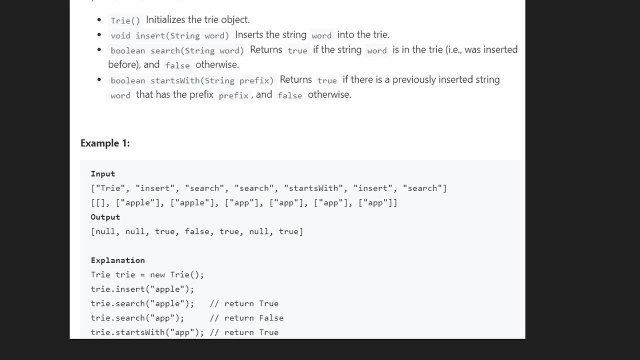 prefix. So those are the three functions we're going to do, And let me just go through the rest of this explanation and then I'll show you what a try actually is. So here you can see basically what we're going to actually be doing. They're going to be instantiating the try, right? We're? 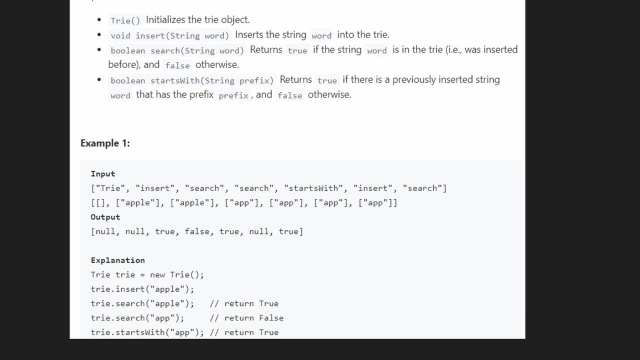 going to be inserting a word such as apple, right. Then we're going to run search: Does the word apple exist? Well, we just added it, So of course we're going to return true Apple exists. Then we're going to check: Does the word app? 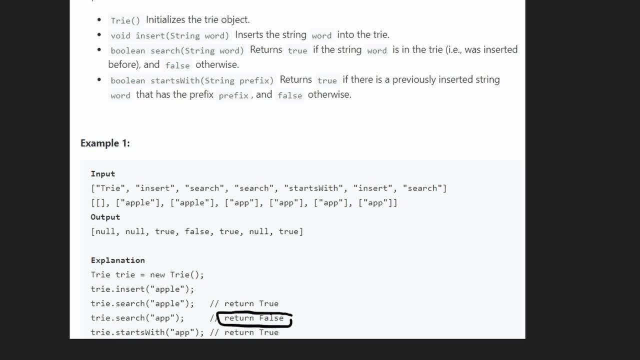 It does not. The word app does not exist. And third, we're going to try: starts with app. Are there any words that start with app? And answer is yes, So we return true. Remember apple starts with app, So we return true. the prefix right. This is the prefix. app is the prefix of apple. 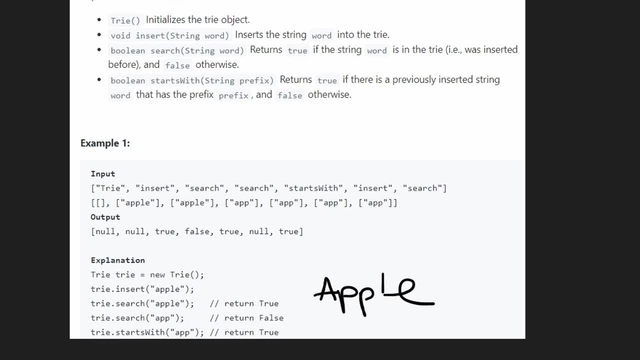 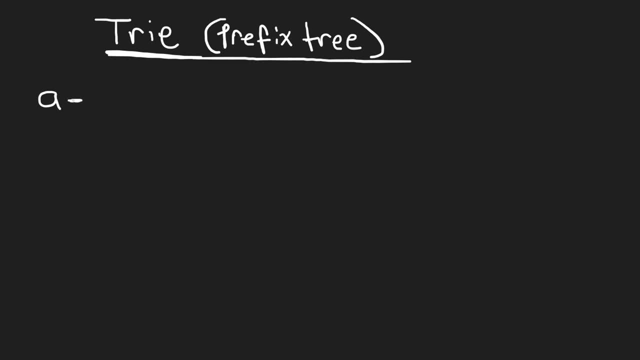 So now let me show you the actual data structure. So let me show you what a try is. And in this problem, they told us that the limitation is that the words are going to only have characters from lowercase a to z. right? So this is a lowercase a to z, So that means we're going to have exactly 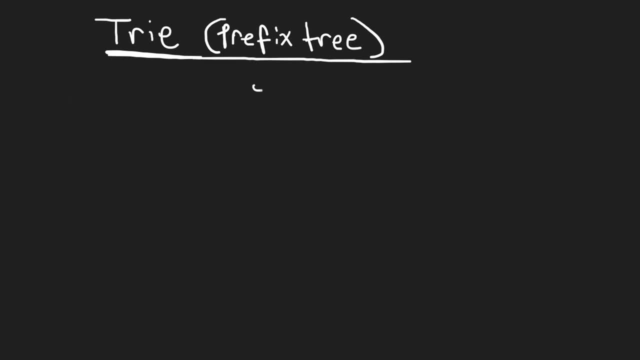 26 characters to worry about, right. But so this is a tree, right, It's a prefix tree, It's a special kind of tree. So initially, our tree, our tree, is going to be empty, right, But let's say we. 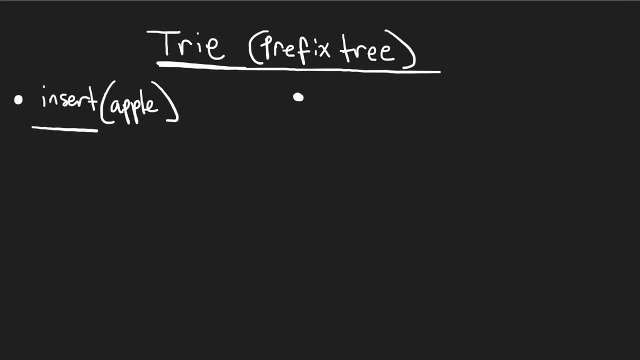 want to insert apple. So if we want to insert the word apple, how can we do that? Well, this is what we're going to do: We're going to create a node for the lowercase letter a right, Then we're going to create another node for the lowercase letter p And we're going to basically 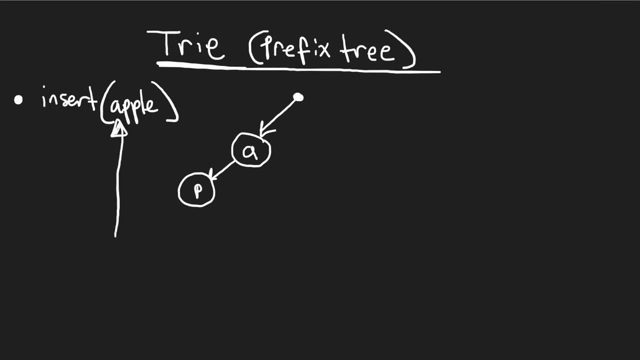 keep doing this for every character in the word that we're inserting right, We're going to say a: insert it p, insert it second, p. keep doing that, And every time we're inserting a new character, we're going to add it as a child. 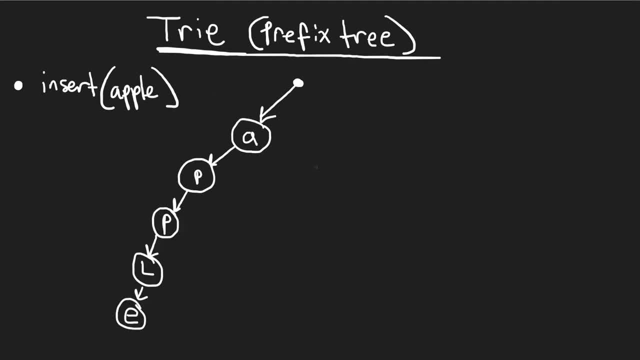 So we inserted the word apple, right, We can clearly see that. One more thing we have to do to say that this is the word that we inserted is we have to mark the end of the word right. So this is the end of the word, right. The letter e is the end of the word, So we're going to mark it. 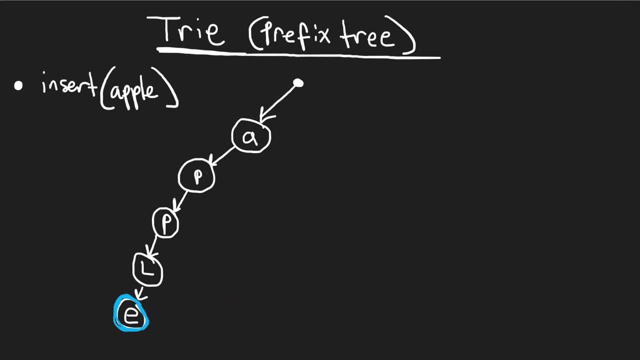 such that, so that this is identified as the end of the word right, Not, for example, this right. If we mark this as the end of the word, then we're basically saying we inserted the word a- p, but we know we actually did apple right Full on apple. This is the last character. 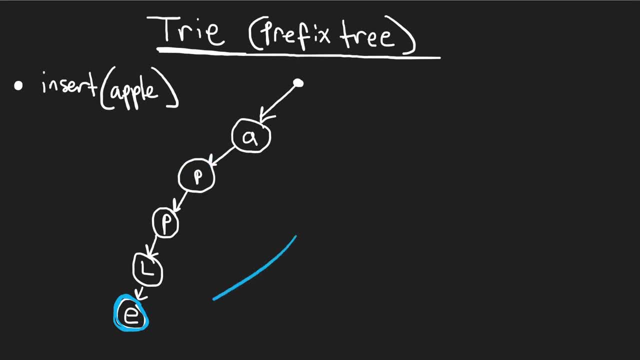 So we mark here as the last character. We are marking it even though it's kind of self explanatory, because this character e does not have any children. It's basically obvious that this is the end of the word, but we're still marking it just to be safe. So you can kind of 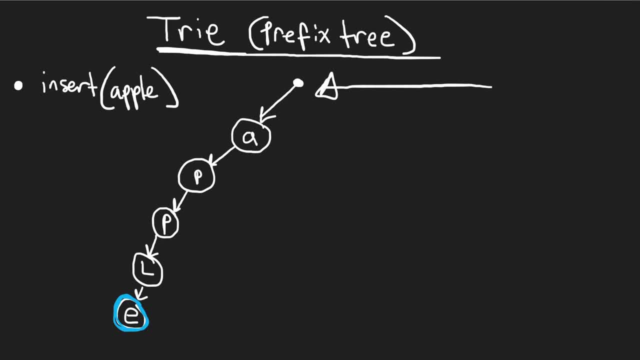 see what we're doing here now, right, This is kind of the root, right. So really, what's going to be possible is we have 26 characters, right? So potentially we could have a node at the first layer for every character, right? So a, b, c, d, etc. right. 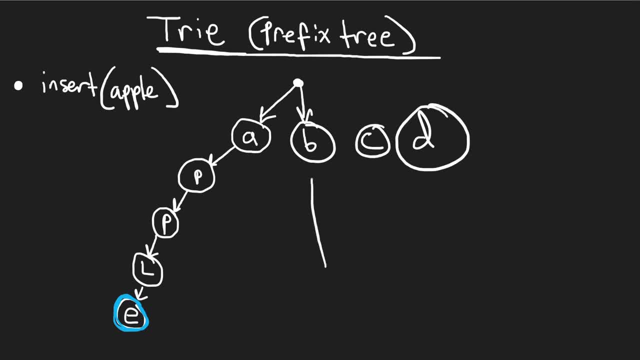 We can have a node for each of these, basically indicating that here is where we're going to put all of the words that start with a, b. Here we're going to put all the words that start with a- c. Here's where we're going to put all the words starting with d. So the next thing we're going, 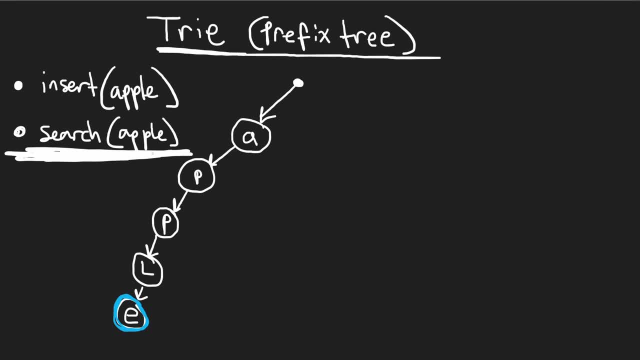 to do is run search. We're searching for the word apple. So how are we going to do that? Well, we're going to start here, at our root. right, This is technically our root, even though it doesn't really have a character. right, So that's basically just a placeholder node. right, It doesn't have. 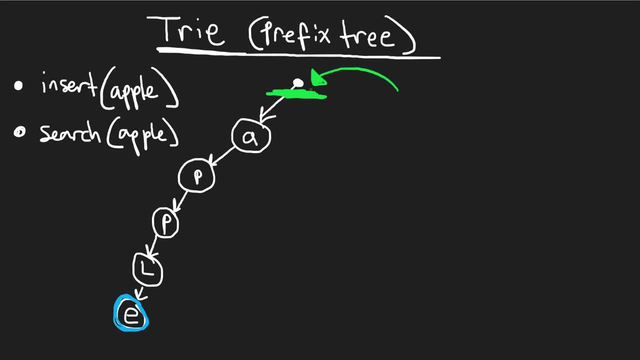 any characters, but it's considered the root, right? And so we're going to check. does this root have the child of the first character that we're looking for, right? So take a look, This is the word we're looking for. Obviously, we're looking for the character a, So we check, hey. 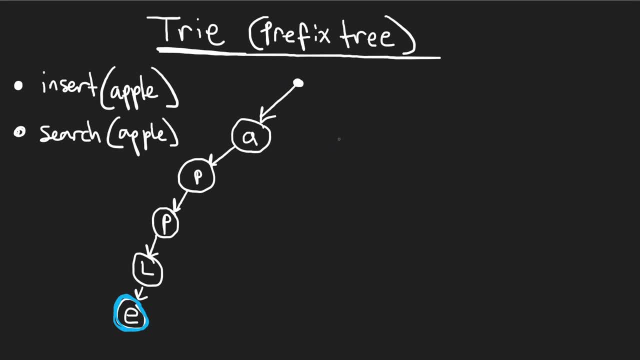 there's the a lowercase, a right. It's the first character of the word. That's what we're looking for, Great. Now for this, a we're looking for the next character, right. So does this? a have a child. 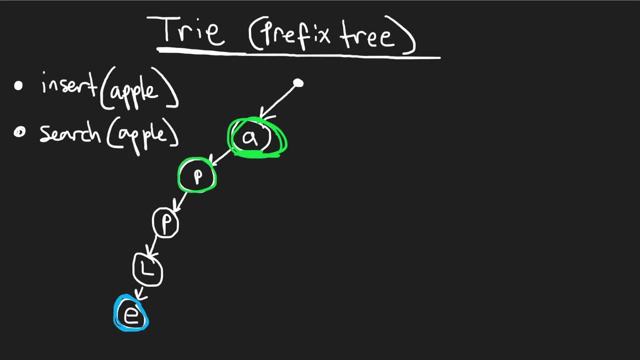 p character. It has exactly that. So we do have this p right. And this is what we're doing right. We're going character by character in the word, we're searching for and checking if a node exists for each character consecutively, right As a child. So next character p does this have. 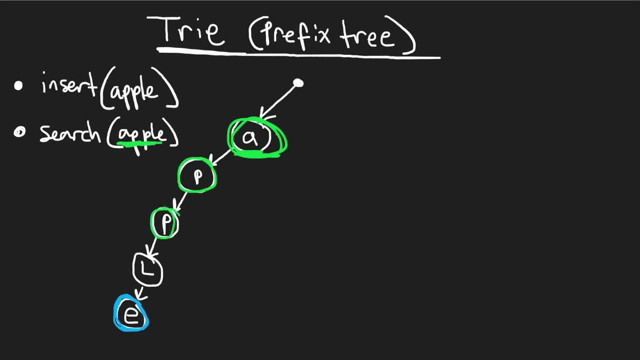 a child p: Yes, it does. Next character l: we have a child l. Next character e: this is the last character, So we do have an e And last thing that we have to confirm is: okay, this is the last character. Is it marked such that? 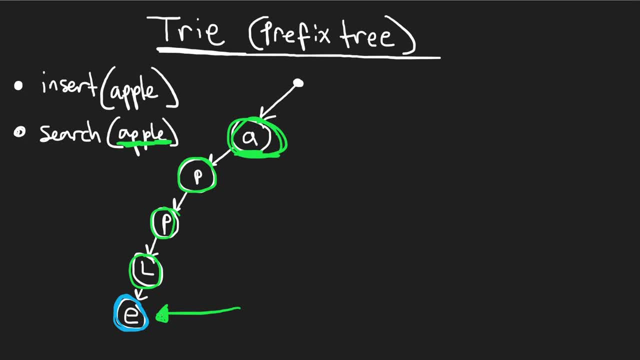 this is the end of the word. Is it marked as if it was the end of the word? It's blue, right. That's what we're doing to indicate that it's the end of the word. So it is right. So clearly. we do have 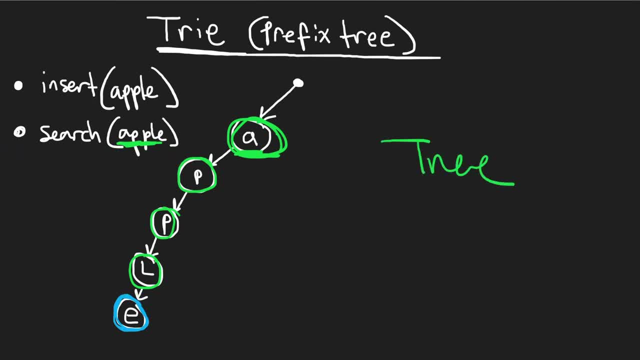 apple. We search for apple. What do we do? We return true because apple does exist in the try. So next let's run search again And this time let's check if a word app exists. So we do have apple inside of our try app, right, Not apple. So obviously we know that starting. 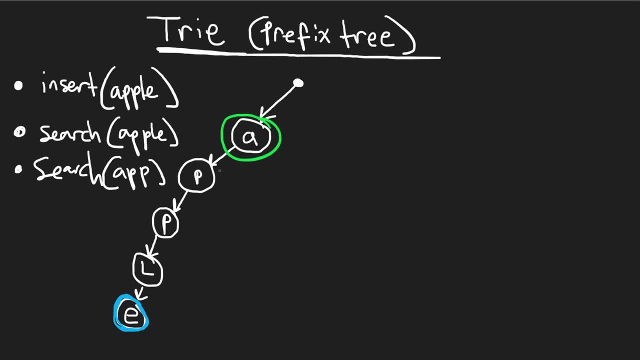 from the root again. we do have a lowercase a, just like we checked. We do have a lowercase p after that And we do have a second lowercase p. So since we do have all three of these characters right- A, p, p- Shouldn't this function return true? No, we're not returning true, And the reason? 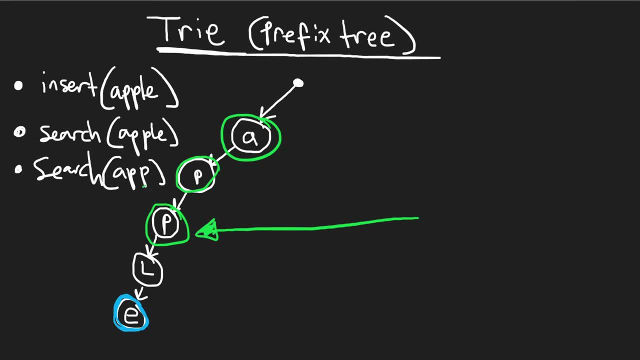 is. this node is the last character of the word, right P And it's not marked blue, meaning it's not marked blue. So we do have a lowercase p after that And we do have a second lowercase p. So remember, we only inserted apple into our try, right Into our tree, And we marked this as the 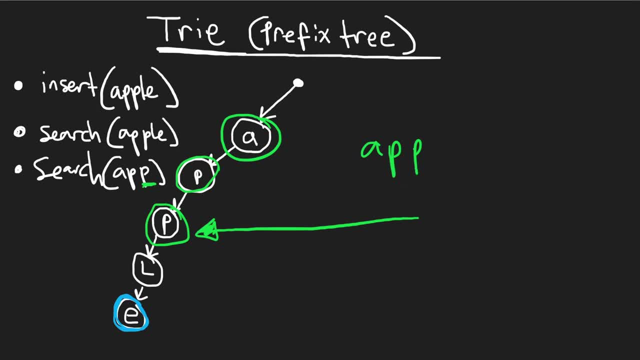 end of the word. We never inserted app into the tree, So this is not marked as the end of the word. So we return false for saying that app does not exist in our tree. App is not a word yet. Next let's run another function on our tree or try. We're going to check. does a word start? 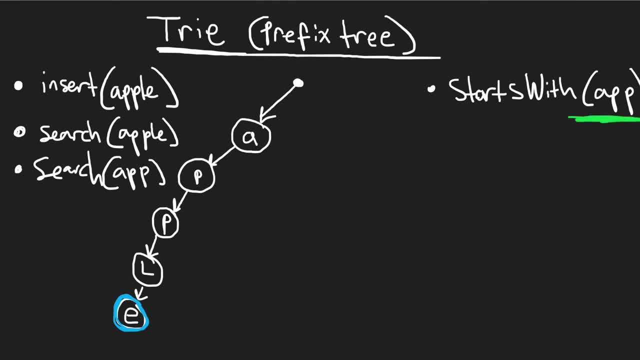 with app. How can we check if a word starts with app? Well, we're basically running the exact same thing that we've done, right? We're starting at the root. We're going to check character by character. So this is pretty like. all three of these functions are pretty similar, right? We're? 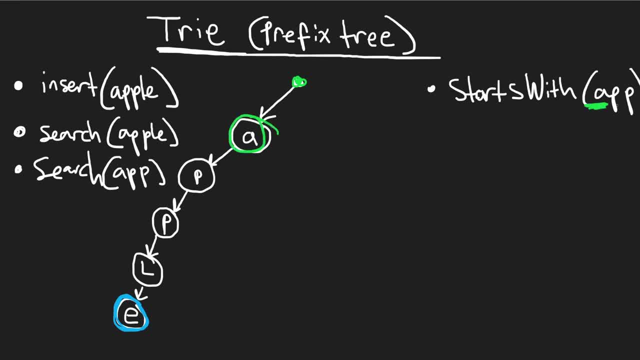 checking character by character. for all of them Start at a: a exists- Check p. p exists. Check another p: p does exist. So since we found all of the characters right, We're basically guaranteed that either this is a word itself or it's not. So we're going to check character by character. 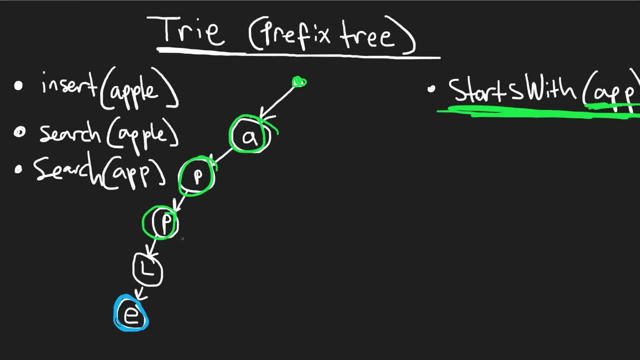 Which clearly it's not right. We never inserted app, or we're guaranteed that there is some word below that has been marked right, Because if we inserted these characters, we only did that because we were inserting a word, So there's guaranteed to be at least something that is. 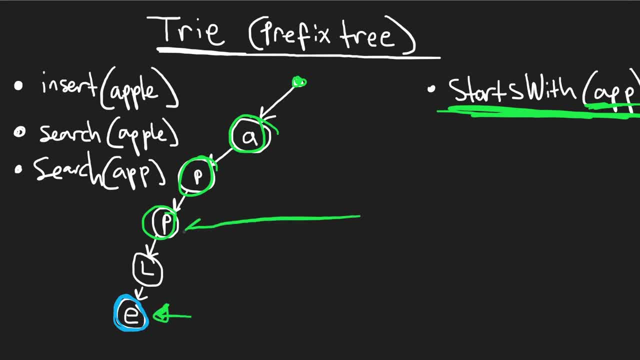 marked blue down here, right, So? so once we found this character, the second p, which is all the characters in here, then we can say true, right, There definitely exists a word that starts with app, right, And so this starts with function, right. So we're going to check character by function. 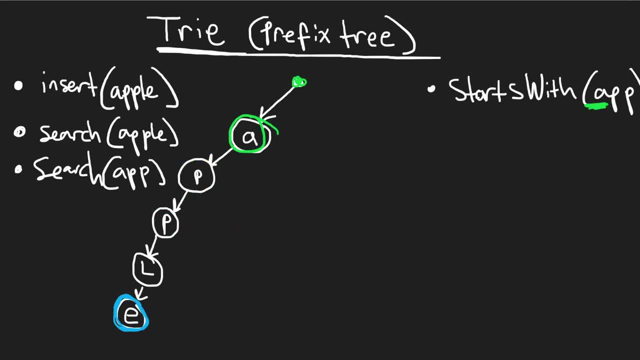 Is the main reason we're even implementing a try in the first place, because if we want to insert words and search for words exists right To check if a word exists. we could just use a hash map for that right, Because hash maps can, or hash sets can, do both of those things in O of one time. 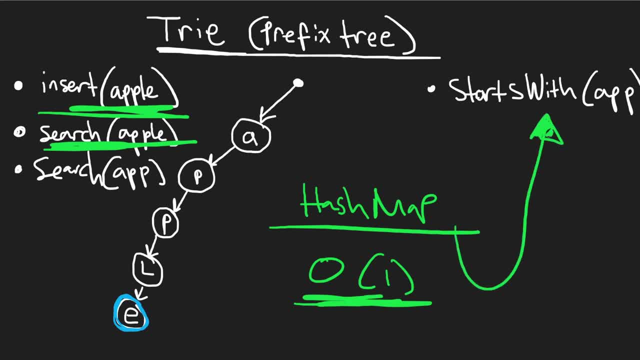 right. But this is really the problem starts with. it allows us to check prefixes, right. So now let's say we were inserting another word. Let's say we're inserting the word ape, right, A, P, E. how are we going to do that? Right, We're inserting another word. What does that mean? Are 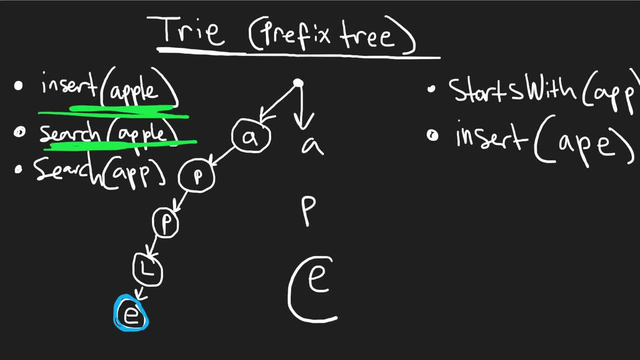 we going to say a, P, E, and then just create a separate node for each of these as children, right, And just connect them, such as that right: This is a child of a, this is the child of P. Are we going to do that? No, because we could reuse it right. Why would we have duplicate? 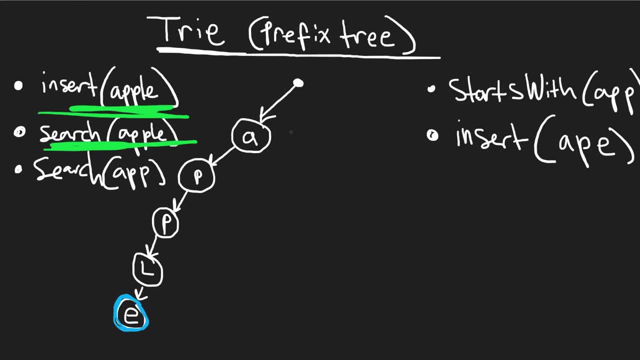 A's in the first position when we already have an A over here. So if we are inserting this word ape, we're going to leverage this A that we already created Great. And then we're we're adding the second character, P. We're going to leverage this P that. 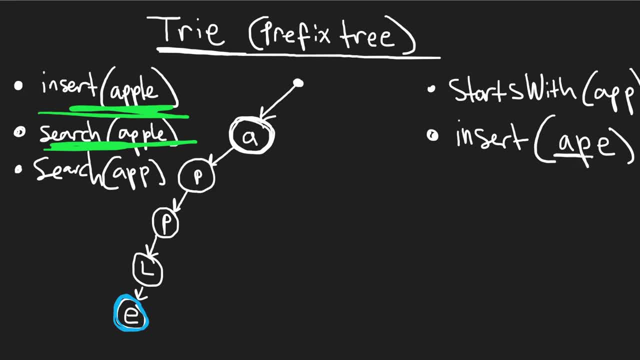 we already created, And so we've inserted the first two characters. What about the last character, the E? Do we have an E over here? No, right, There's no E in the third position. So what are we going to do? We're going to create another child node. right Now, we create an E, and last, 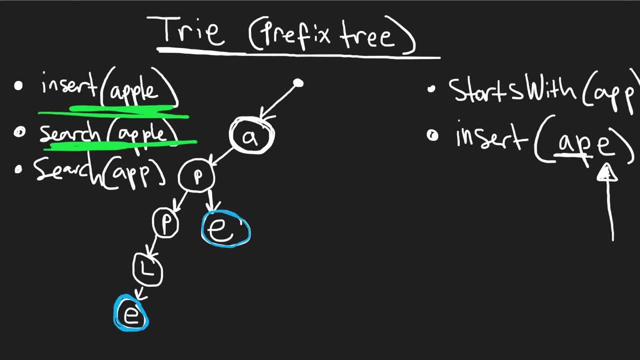 but not least, we mark that this is the end of a word. So you can see that a try actually has a potential To be pretty efficient, because we are reusing a lot of nodes right. We're not necessarily creating a separate node for every single word. Now let me just show you one last thing before. 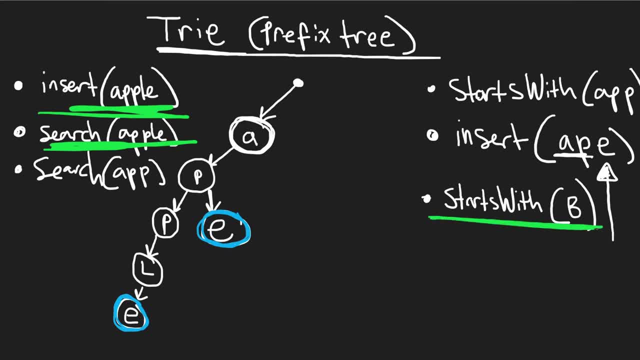 we jump into the code. So we're going to do one last function. We want to check Does any word start with B? and I'm just illustrating why we're even implementing a try in the first place. It's because the starts with function is very efficient compared to other data structures. So, for example, 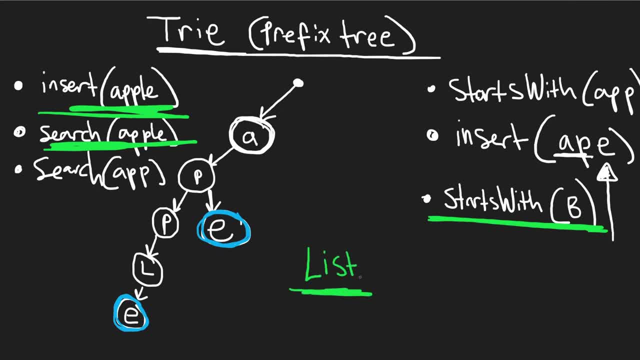 let's say we had a list, A list of words, a list of strings, and let's say the size of that list was equal to a million. right, How long would it take for us to check if any word starts with B? Worst case we would have. 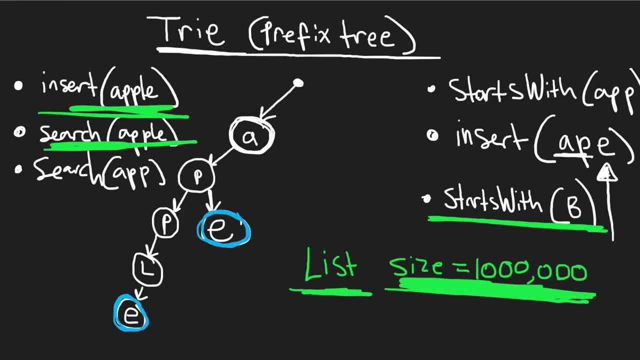 to check every single word in the list and check if it starts with B. and what if there was zero words that started with B? then every time we would have to go through that entire list of a million words. But with a try it's very efficient. Here you can see we implement. we have two words right, We have one. 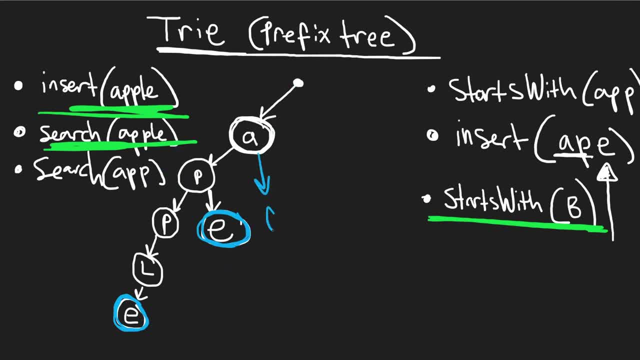 word here, and we have a second word here, and it's possible we could have a million other words. right, Like, clearly, there's probably a lot of words that start with the character a and maybe so on, But when we run, this function starts with B. all we're checking is we're starting at the 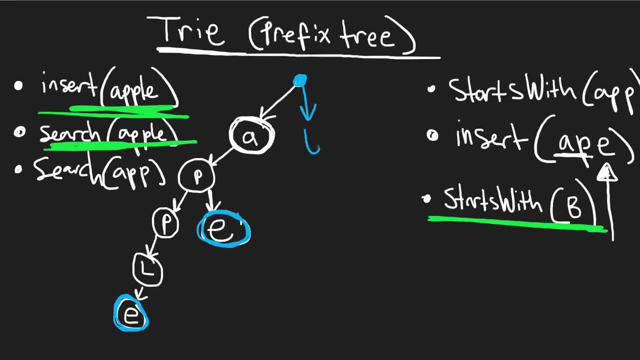 root. We're checking. Do we have any children with the character B? right, We check this first layer. How large Is that first layer going to be? Well, we know that there's 26 lowercase letters, right? So worst case it would be lowercase 26, and that's pretty efficient, right? So when we check, we 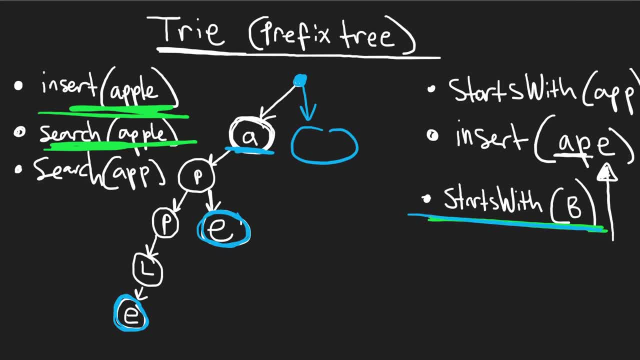 check. Hey, there's a lowercase a, but there's no lowercase B. So for this starts with function. we can return false And that was done very efficiently, right? Uh, 26 is basically big O of one, So this is a super efficient way to uh to check prefixes, right, And that's why they. 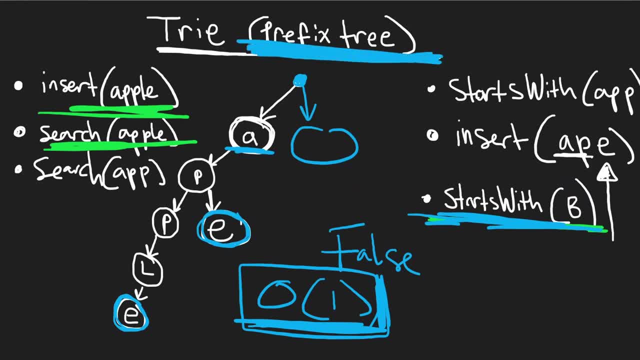 call this A prefix. tree prefixes can be checked very efficiently. So now let's actually jump into the code. All three of the functions insert, search and starts with are pretty similar functions. So the even though we're going to write a lot of code, it's going to be mostly similar. So let's 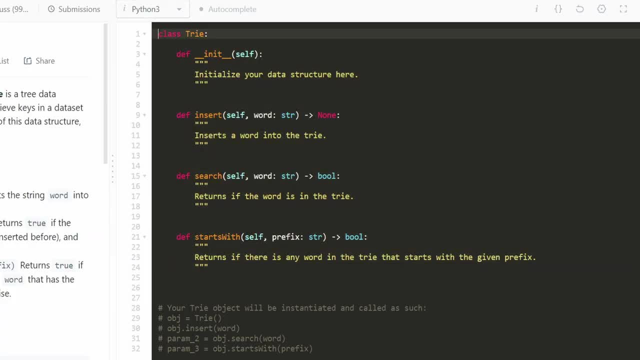 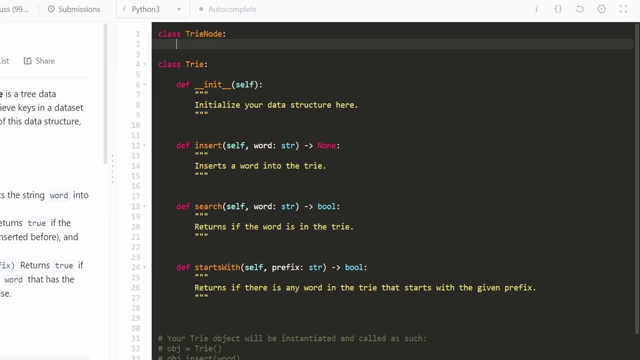 jump into that. So our job is to implement a try, but we can't really do that without implementing a tri node. So the first thing I'm going to do is create a tri node, And all we're going to do is just create the constructor. 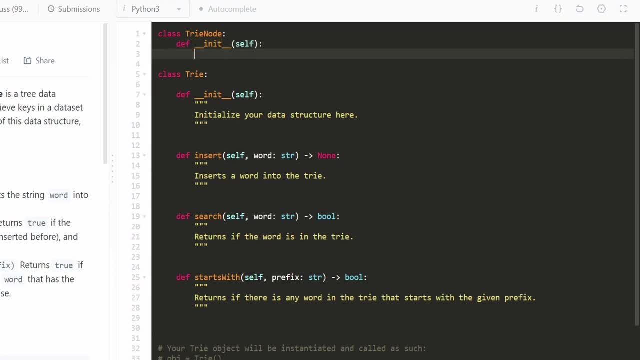 So in Python, that's what I'm doing in net is basically the constructor And I'm just going to have a couple of uh member variables for this. So we are going to have children of a tri node. right, It can have children, It could have 26 children, but instead of doing an array, I'm 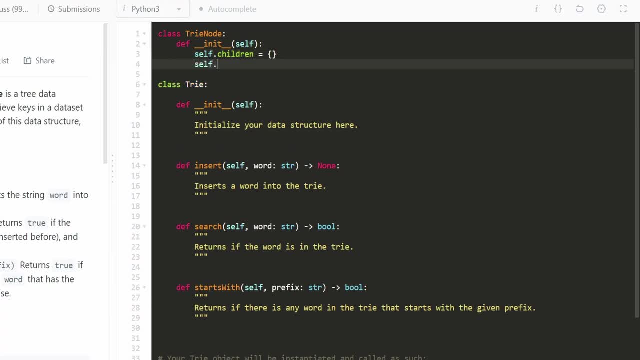 just going to do a hash map because that's easier And remember. we can also Mark every single node as if it was the end of a word. I'm going to say: end of word is going to be a variable. Initially it's going to be false. 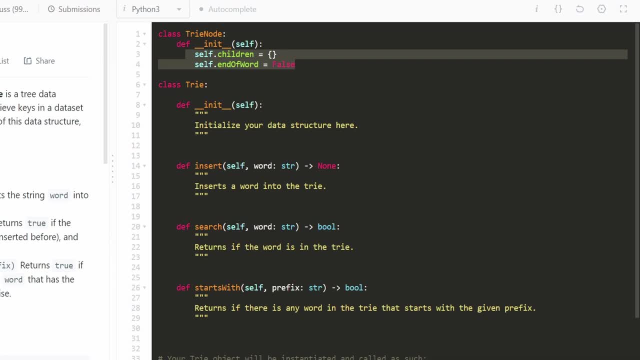 But we could set it to true If the character was the end of a word. notice how we're not actually storing the character itself in the tri node. That's going to be implicit from the hash map, from this hash map. So if we were adding a, let's say, a character, a, a lowercase character, 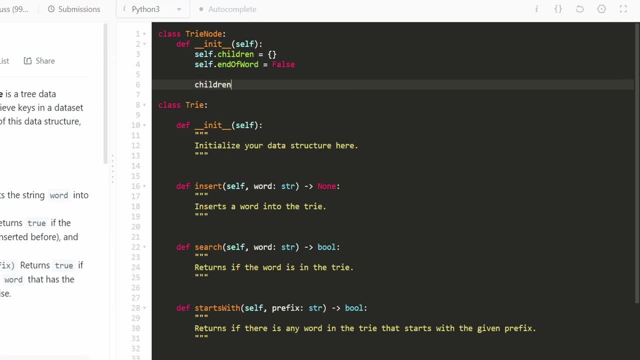 a. we would say to children. we would say children, uh, for character a is the key, And we're going to create a new tri node for that character, a right. So that's how we're going to be doing it. That's how we're going to be. 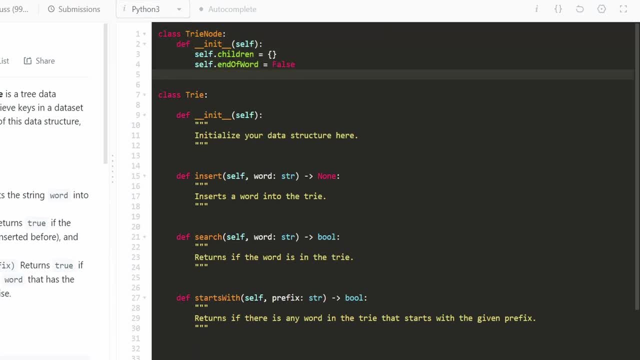 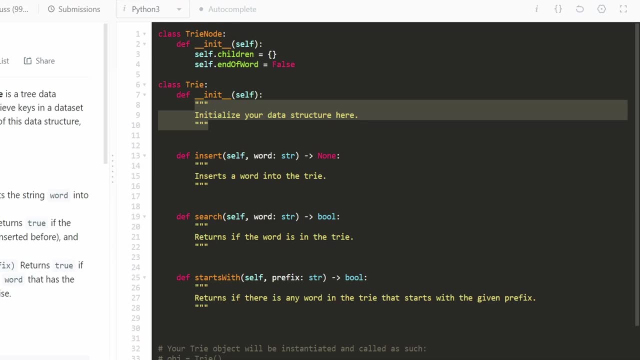 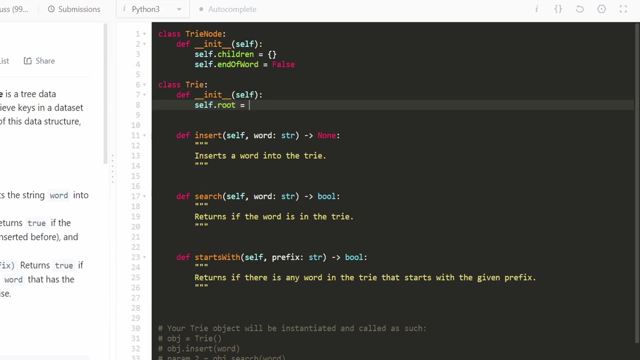 Reserting a node. So that's our entire tri node class. Now let's actually get into the tri class. So the first thing we're going to do is initialize this. So let's get rid of this comment. And for initializing this, all we're really going to need is a root node and we can get the rest of the. 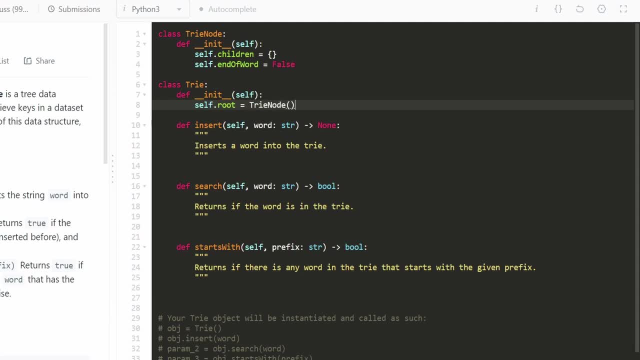 nodes from that root. So we're going to create a root tri node and that's it. That's all we're going to do for the constructor And once the tri node is created, we basically have an empty tree. we have a root, it's empty because it does ha. it does not have any children, So we technically have 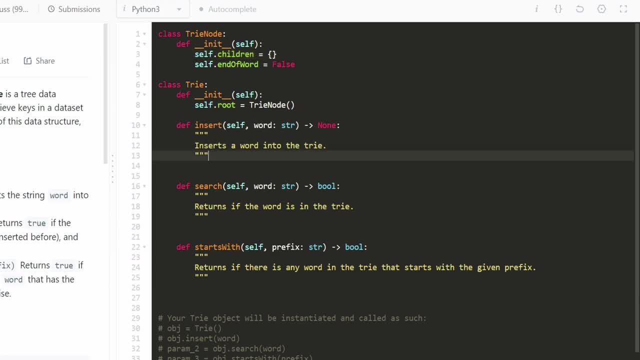 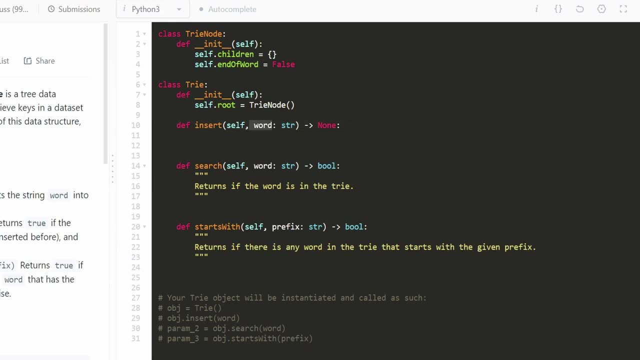 not inserted any words yet, but now let's implement the insert word method, This method for this method, we are going to have to iterate through every single character in the word, So we're going to initialize our self. current is going to be set to the root, So we're going to initially. 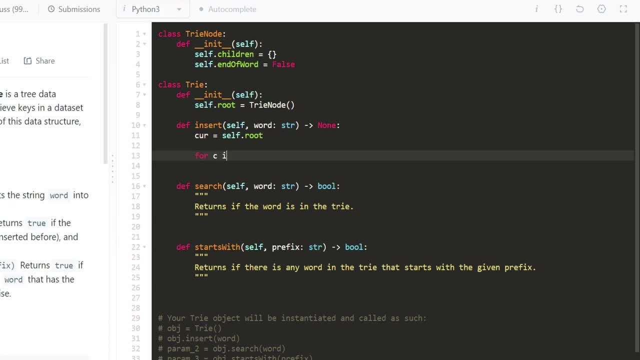 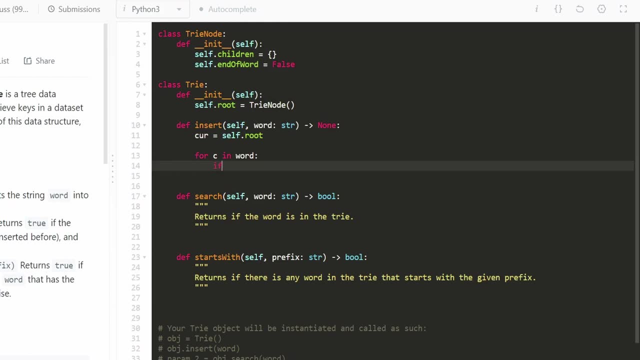 start at the root right And then we're going to go character by character in the word, And for every single character we're just going to check two things: Does the word all? does this character already exist? If it doesn't already exist, So if this. 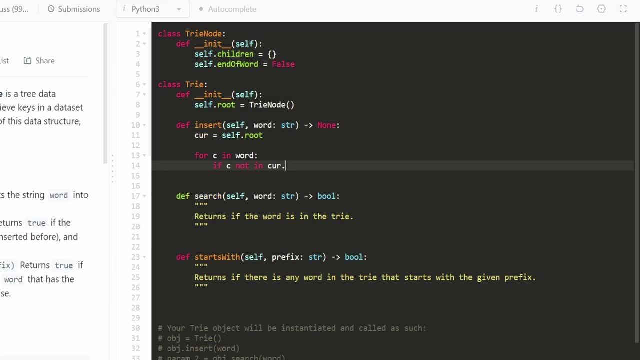 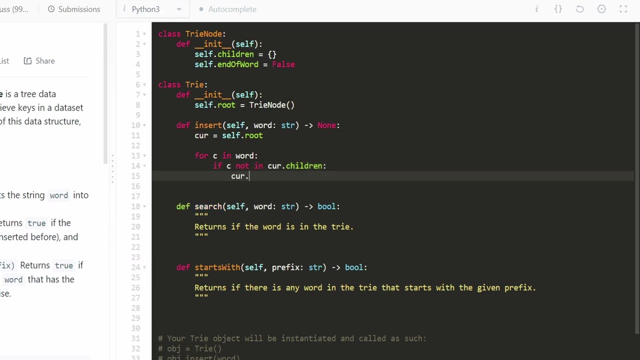 character is not in the current nodes: dot children hash map, right. So if the current, if this character is not in our hash map yet, that means it's hasn't been inserted yet. So what are we going to do? We're going to create a tri node for this character. So cur, dot children. 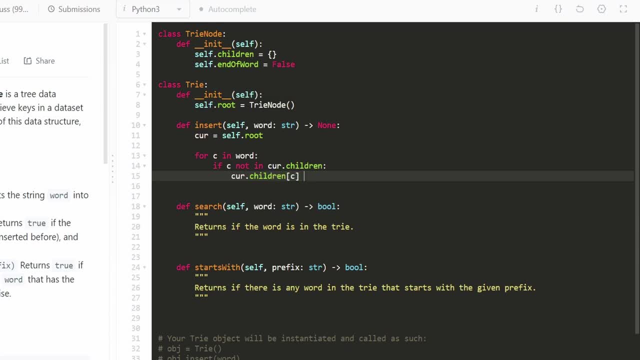 and the key value we're going to use is the character, And then to create a new tri node. so this is how we are going to be inserting characters to children: we're going to use the character as a key value and then we're going to create a empty tri node. 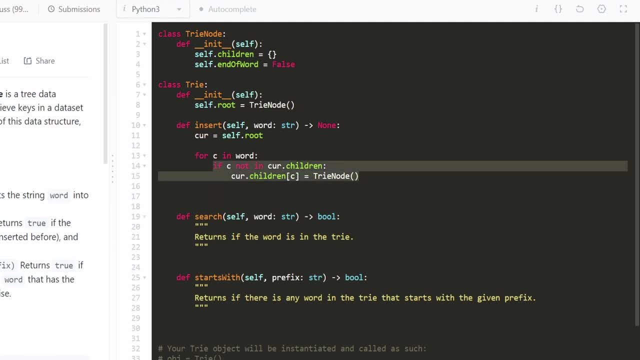 and we're only doing that if the character doesn't already exist. if it does already exist, then we can skip that step and just say that current is going to be set to that child right. so if that character already existed, then we can just update cur and move to that character and then continue our for. 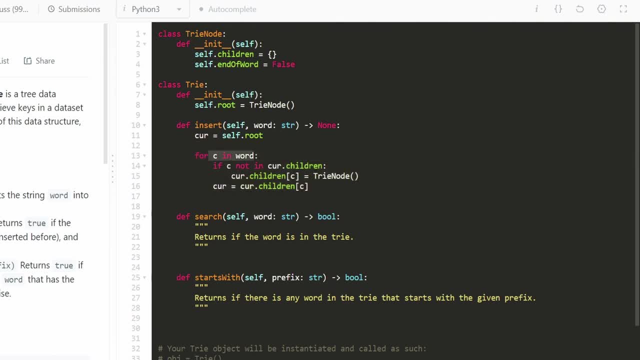 loop, right? so we're going to do this for every character in the word and then, by the end of this loop, whether we have to create every node or the nodes already exist for us. for this word- right, let's say it was apple or something- the characters already exist or we just created them now, current. 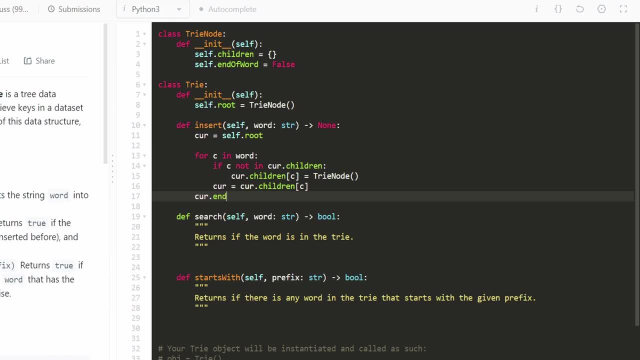 is set to the last character of the word. so what are we going to do to current? well, we're going to mark it as the end of a word, so we're going to set end of word equal to true now, and then we don't really have. 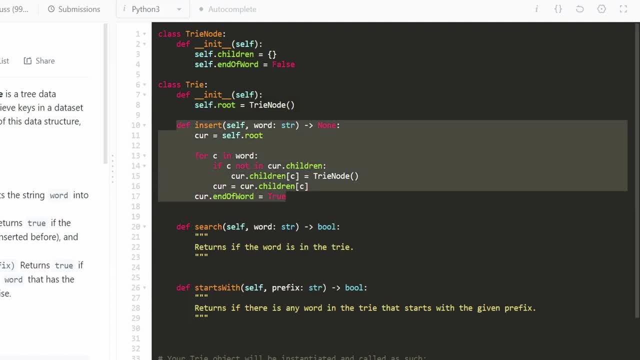 to return anything. so that was pretty simple, right, not a lot of complex code. we did have to go through every character and we either created nodes or just iterated through those nodes and every and the remaining two functions- search and starts with- are actually going to be very 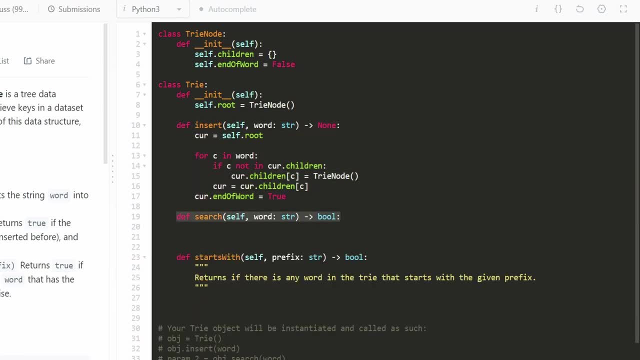 similar to this insert function. so now let's get started on search. so we want to search to determine if a word exists or not. so, just like the previous function, we're going to start at the root node, so self dot root, and we're going to go character by character in the word and we're 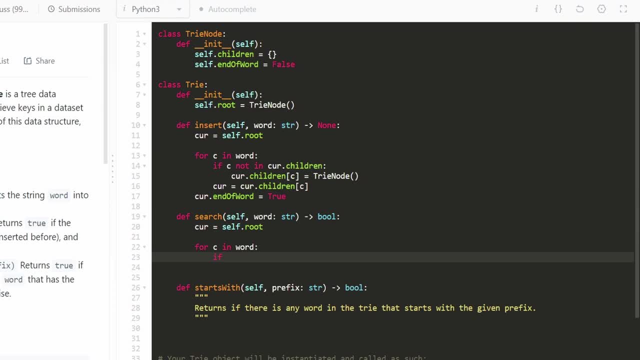 going to check if this character exists in our tree. if it does not, so if c not in current dot children. if this character does not exist, then what do we have to do? we return false meaning. the word just just simply does not exist. if it does, then we can. 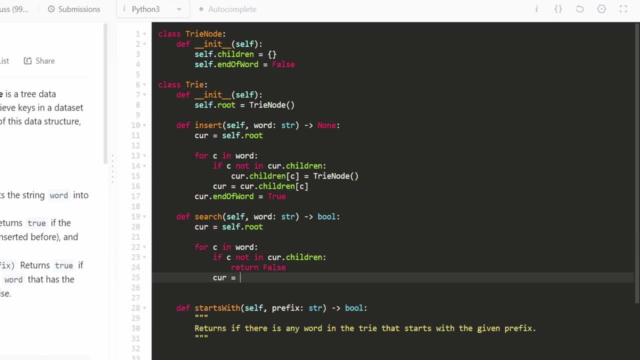 move ourselves to that child node so we can update ker and set it to the child node of that character. and then we're going to basically keep doing this for every character in the word. if the word doesn't exist, we'll return false. if the word does exist, that means the entire loop will execute, and then 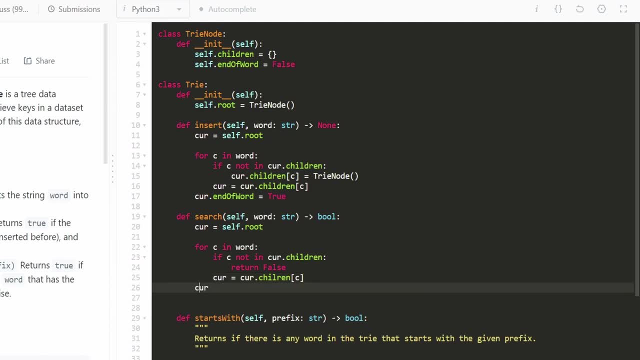 will be. so then ker will be the last character of the word and we- and we know that it is a word- if ker has the end of word variable set to true, so this is the variable we're going to be returning. if this is set to true, that means 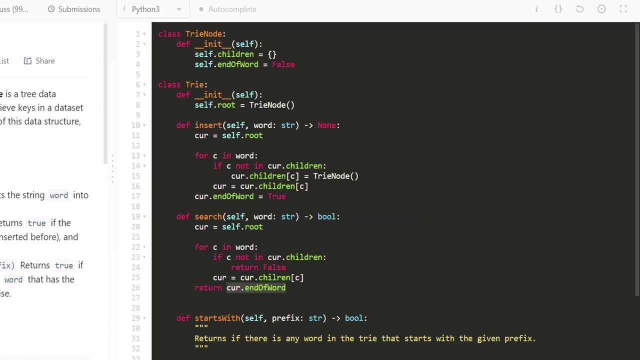 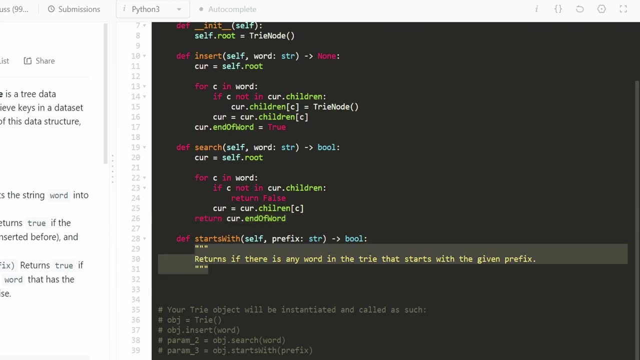 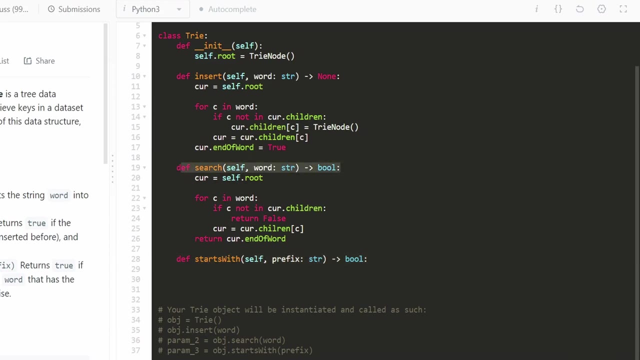 this is a word and will return true. if it's set to false, that means it's not a word and our function is ultimately going to return false. and now, last but not least, let's get started with the starts with function. and this function is actually going to be the exact same as the search function.